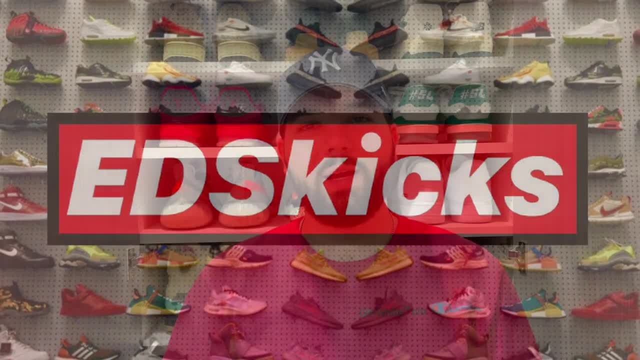 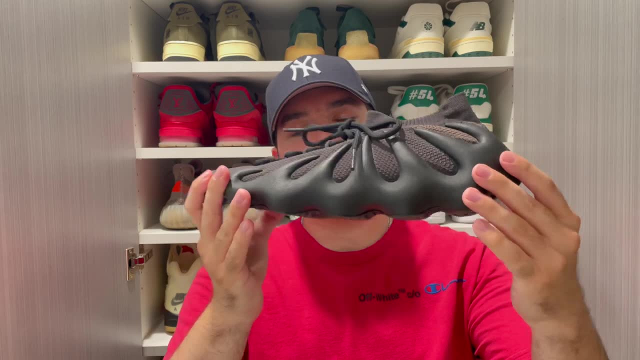 Hey guys and welcome back to the channel. Today I have another update after wear video. This one is kind of a popular one. It's going to be the Yeezy 450 in the dark slate colorway. Now, of course, a lot of people have different opinions on the shoes. Some love it, some hate it. I actually 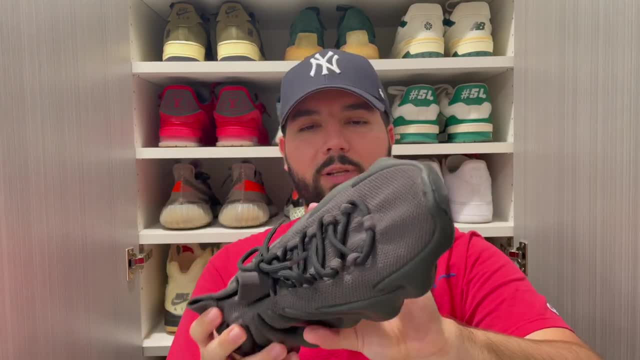 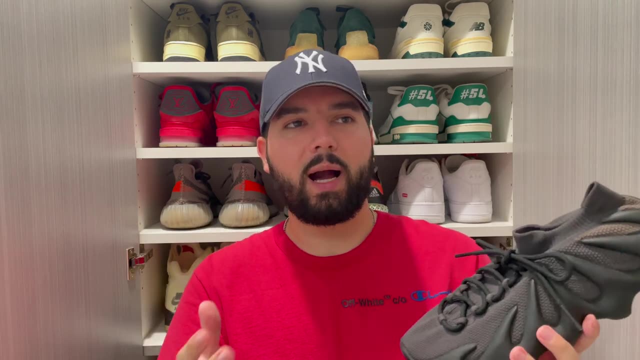 really love these shoes. I think they're, you know, really comfortable and unique and definitely an eye catcher. But what I want to do in this video is not really a review, but more so an update after two weeks of wear. So I just want to discuss things that I wanted to know about the sneaker. 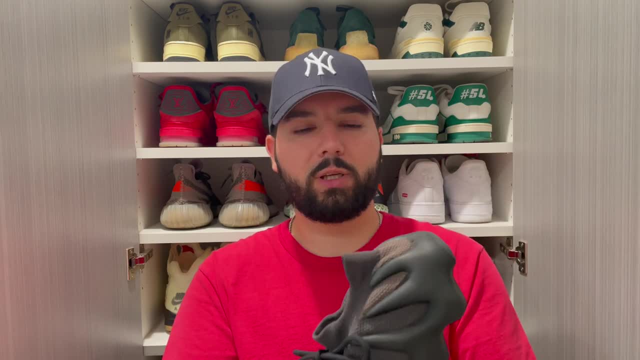 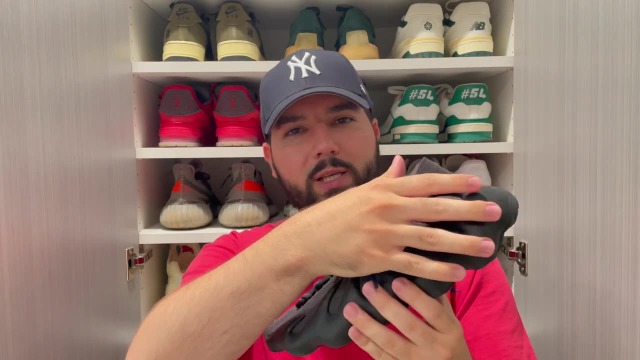 prior to purchasing it. So if you guys are still looking to purchase it, then you can make up your mind, or if you have the pair you haven't worn it yet, then you decide to wear or sell it And I will get into an up close look at it to show you guys some of the wear on it and talk a little bit more. 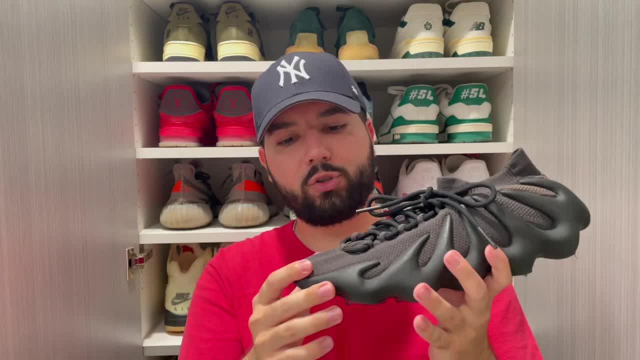 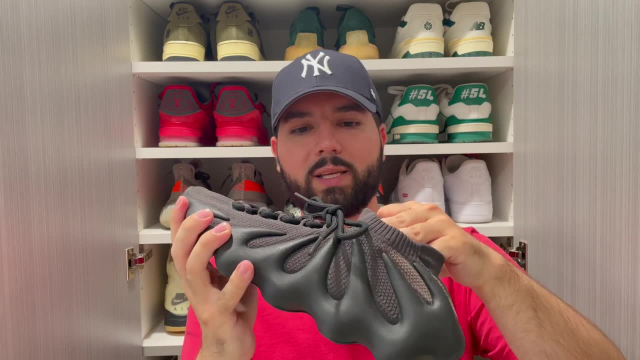 in detail, But in general I really love them. I think they're super comfortable. They are a lot more comfortable than they look. I know this part looks, you know, stiff and sturdy, but it holds up nicely, like you're not going to injure your foot in these or anything like that, But they are soft. 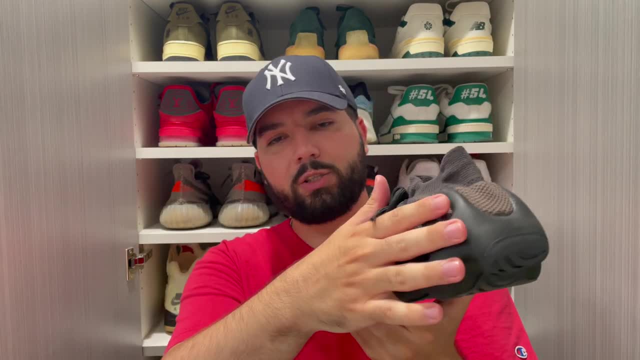 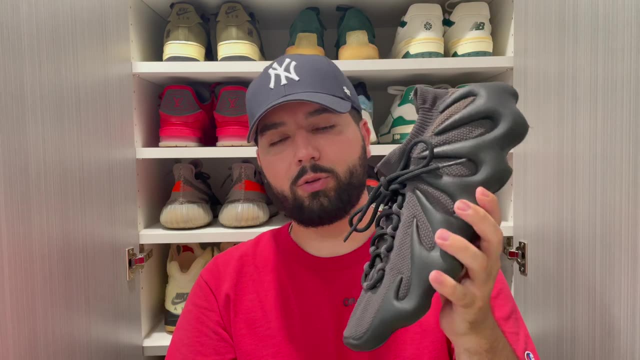 They're very cushiony. so although there's no boost in the sneaker, this cushioning is very soft and very comfortable. You don't feel it bothering your foot at all. Now I am going to talk about sizing a little bit later. They do fit very snug, so you definitely 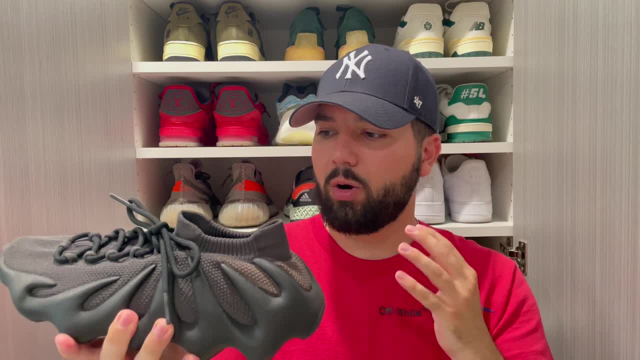 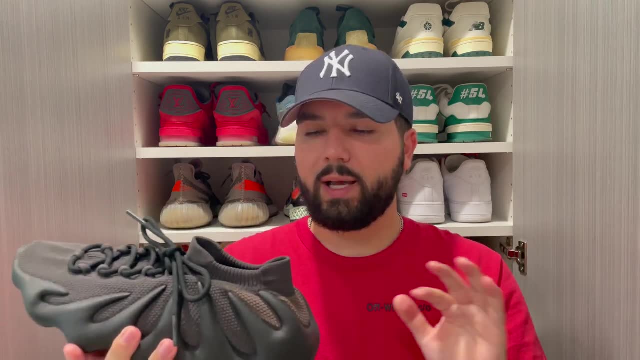 want to pay attention to the sizing portion of this video. Durability wise, they are very durable as of now. They do have some concerns. I will discuss later that might be a potential issue in the future. But as of right now, zero issues. Very glad about that. I don't really expect any. 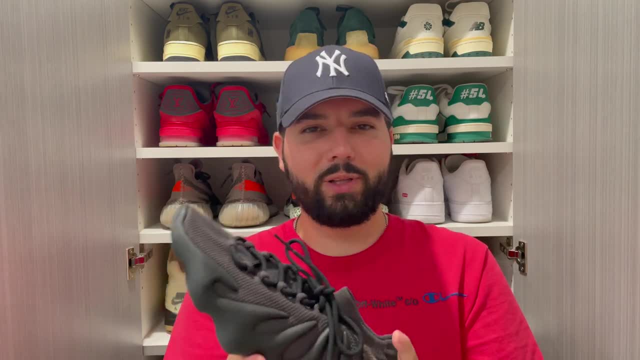 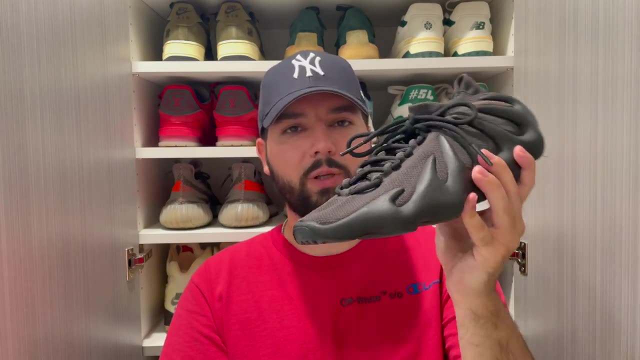 issues with this shoe. you know two weeks in. But you know in knit materials you don't really get any creasing and stuff. so the sneaker looks brand new for a long time. So it really starts wearing down. It's very easy to style. actually It goes with a lot of different. 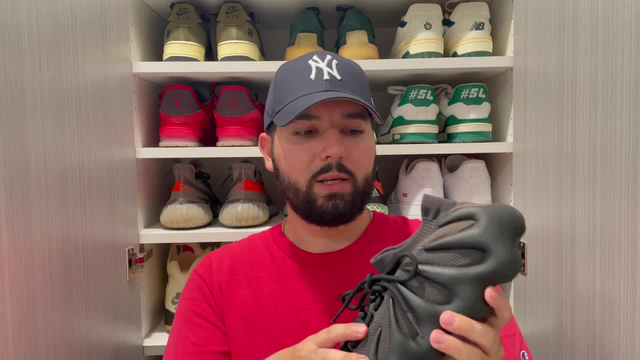 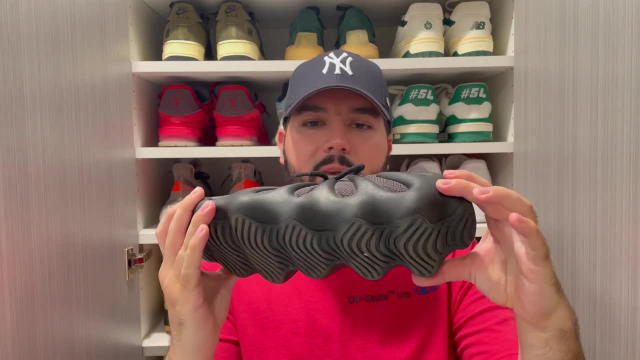 colors, A lot of different types of pants, shorts, you know, socks, So that's a really big bonus on this. You can just slip it on and wear it Really easy, really comfortable and it's definitely an eye catcher. A lot of people are going to ask you questions on what this shoe is, especially if 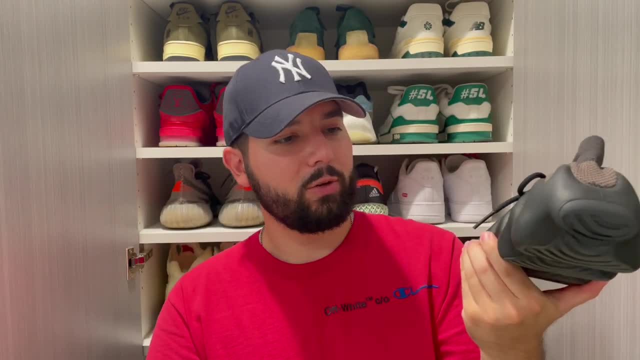 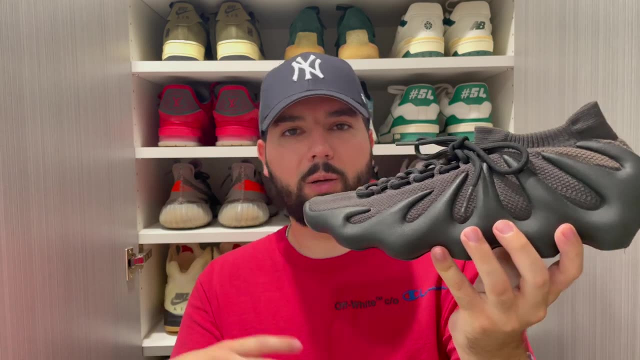 they're not, you know, really sneaker heads or into the sneaker game like that. So definitely a nice conversation piece as well. So, with all that said, I do want to get into an up-close look at these shoes. I guess a little bit of the wear and then talk about sizing and durability. 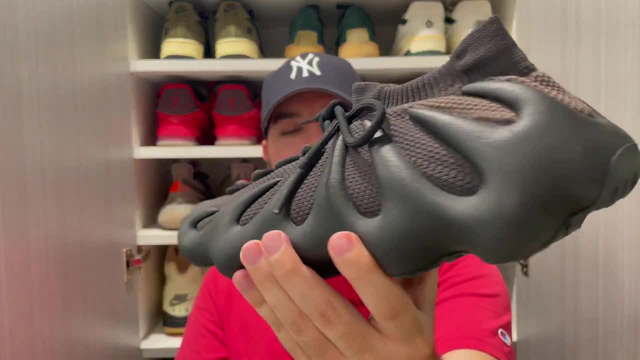 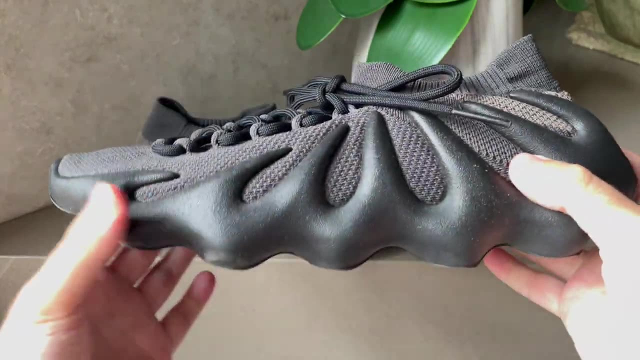 And all that good stuff. Let's get right into the closer. look at the ZZ450 Dark Slate. All right, here's an up-close look at the ZZ450s, So let's just take a quick look at it, See how it's holding up. Obviously I haven't worn them enough to see any structural damage or anything. 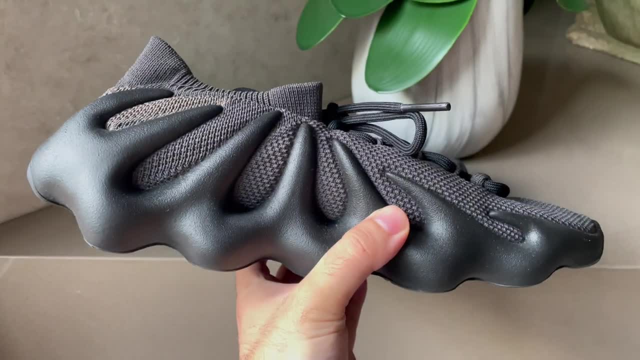 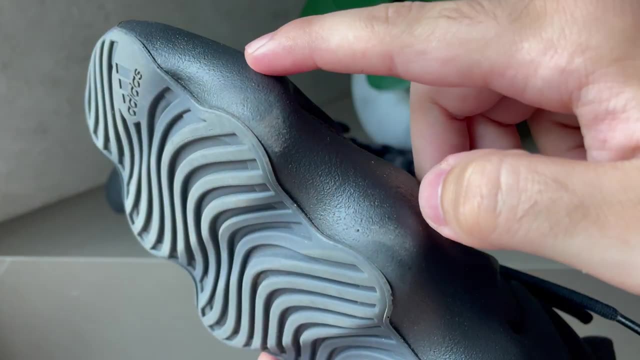 like that. But I still want you guys to see a little bit of wear and where it actually shows. So when you wear the sneakers, you guys could see on these little pods right here you do see the dirt marks, So you're going to see that. But this material overall is super easy to clean. I just 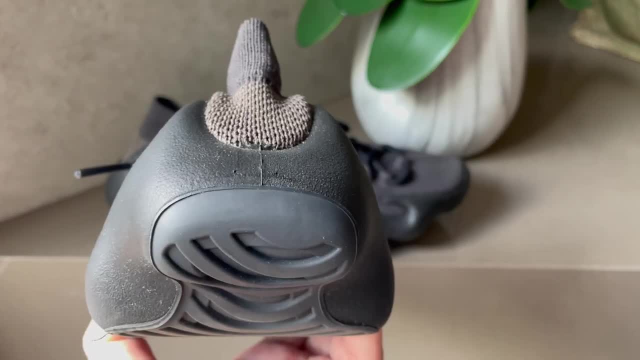 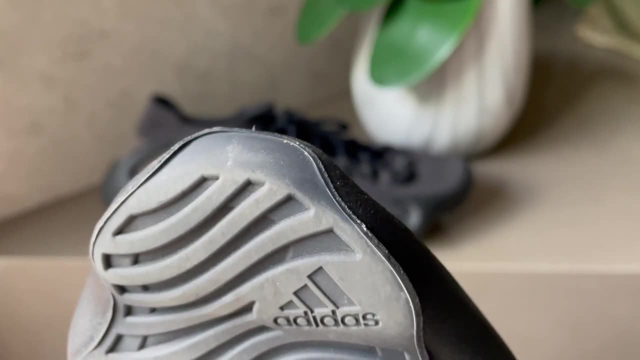 didn't clean it so you guys could see where the dirt marks actually show. Of course, on the back it's kind of a lifted back so you're not going to get too much heel drag over here. So that's a good thing. right there On the front we will get some drag over time. You're already starting to see it. 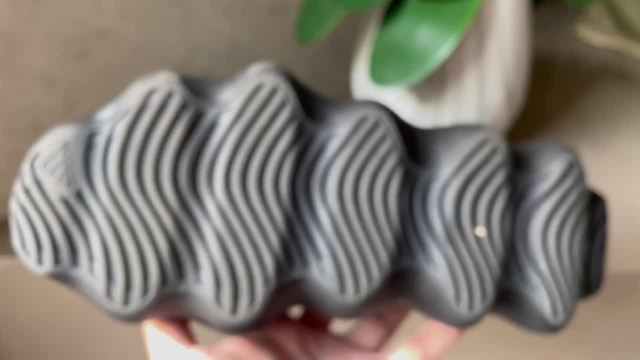 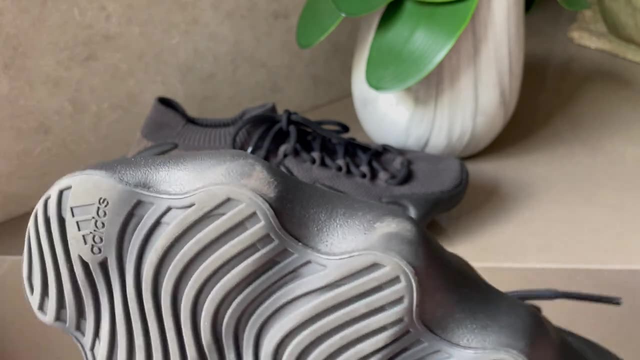 happen a little bit. Let's take a quick look at the outsole. Really nice traction on these, of course, And yeah, it just shows a little bit better. But basically, this is where, like, the dirt marks are going to basically show most of the time. That's where it really touches the ground. It'll probably 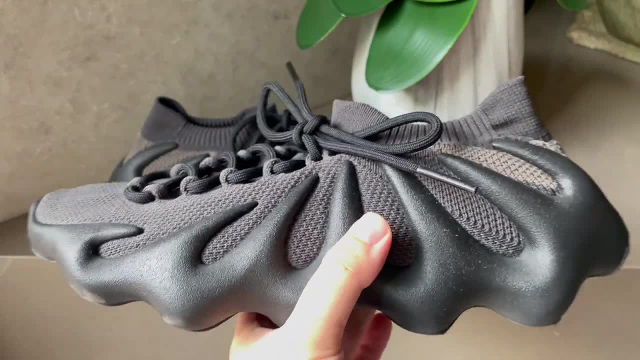 get scuffed, It's not going to look too bad And from far you probably aren't going to see too much. So let's take a look at the outsole. So let's take a look at the outsole. So let's take a look at. 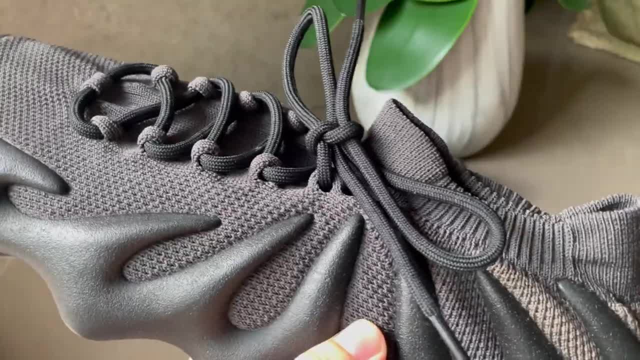 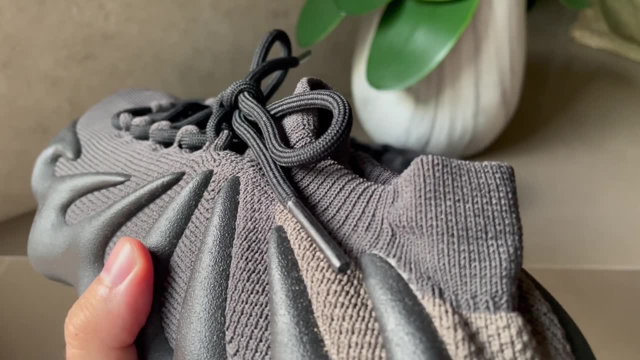 only thing I'm a little bit concerned about over time, If it does happen, is if we start seeing these separate a little bit from the knit. These are basically attached really firmly to the knit, so it's probably not going to be an issue, But after a while, if the knit rips a little bit, this 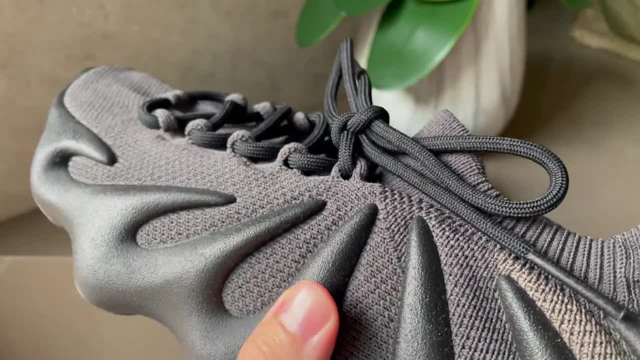 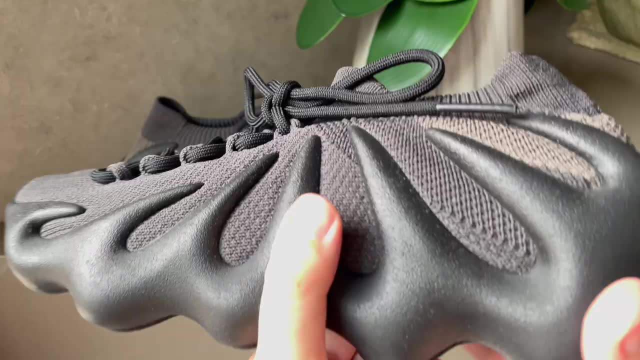 could start, you know, kind of losing its attachment to it and separating. But that's a long-term issue, of course. after just a couple weeks or even a month, something like that of wear, that's not going to be a problem at all. One thing I want to mention with these- actually after wearing- is that they 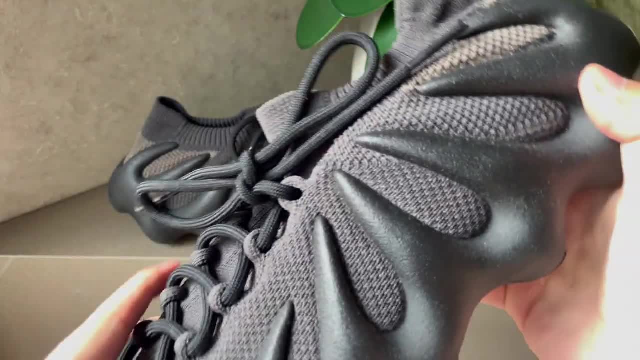 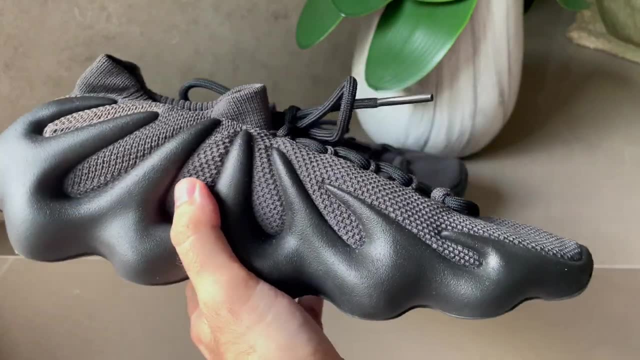 actually don't have a lot of dirt on them. So they don't have a lot of dirt on them, So they actually mold your foot really well. If you guys have watched review videos on these, you know that they fit really snug at first. I would recommend getting a full size, up from your regular size and 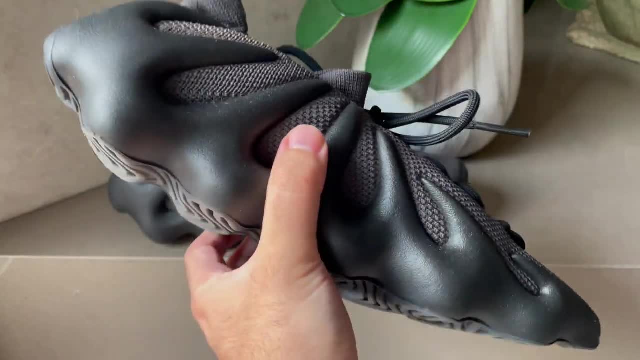 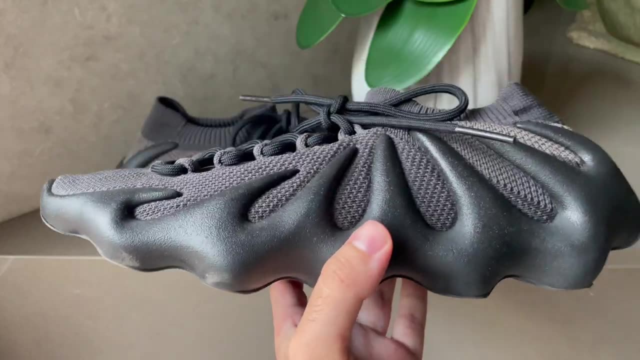 compared to easy 350s, I would go half a size up. I got a size 11 in these. Usually I wear a 10 in most sneakers and a 10 and a half in 350s. I could even honestly fit an 11 and a half in these if I. 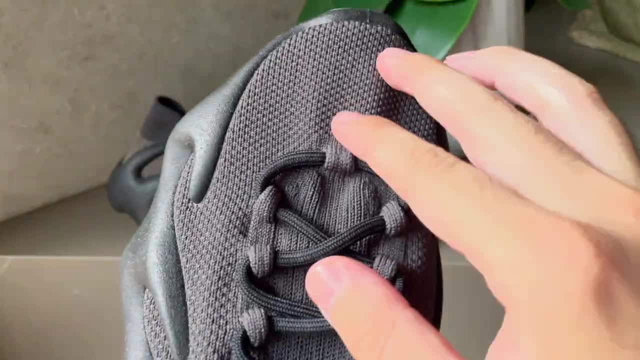 wanted to. That's just how tight they are, And the private material itself is really tight, and they have laces on as well. So I would recommend getting a full size up from your regular size and compared to easy 350s. I would recommend getting a full size up from your regular size and compared to. 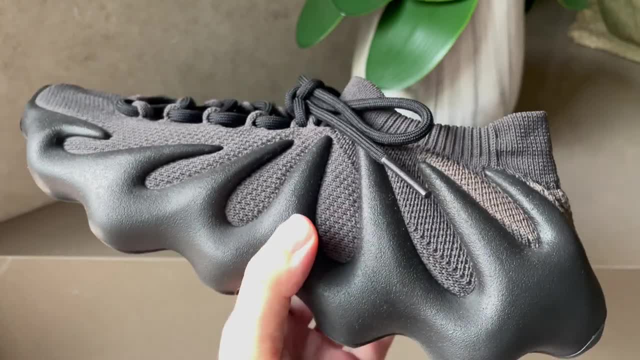 easy 350s. I would recommend getting a full size up from your regular size and, compared to this sneaker fits like a slip on sneaker with added laces, I'll put it that way. So it's definitely a very tight fit and you definitely, definitely want to get your sizing correct with. 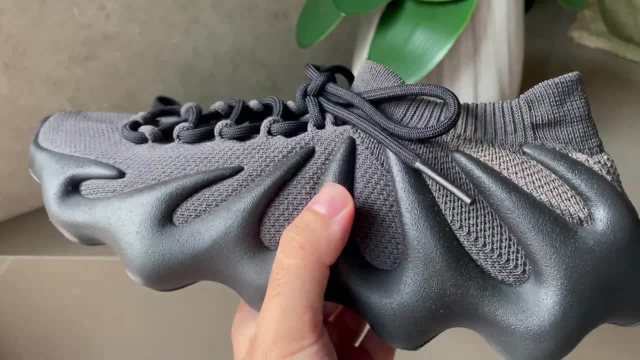 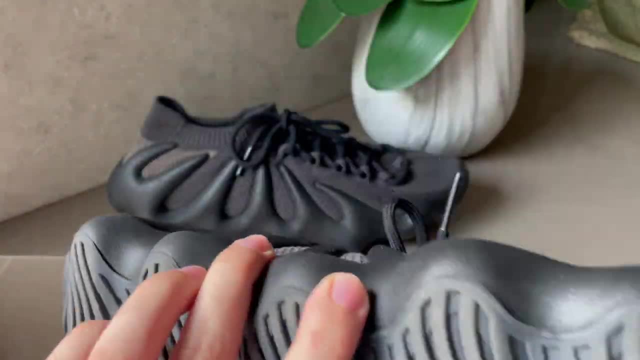 these, But overall, after you start wearing them, as I said, the knit stretches a little bit and molds your foot and they're actually very comfortable. These are one of the most comfortable sneakers I own. Depends on your foot, honestly. Some people might not feel that way. There's no. 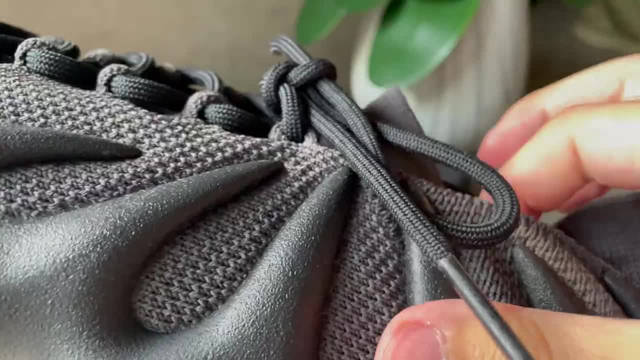 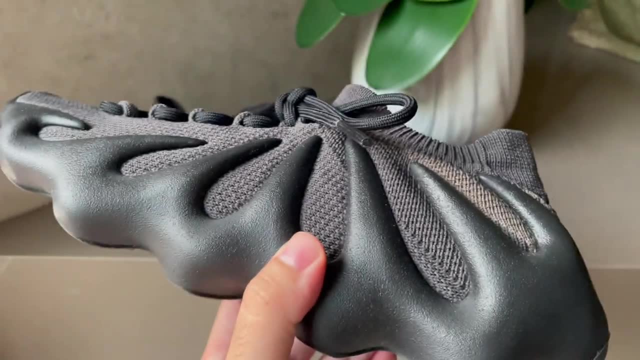 boost in these, but it's actually very soft material. Some of the pictures that might look a. as you guys can see, it just bends super easily. so it's a soft, cushioning material. it feels really great on feet and you don't notice any of this restricting your foot when you're wearing it. 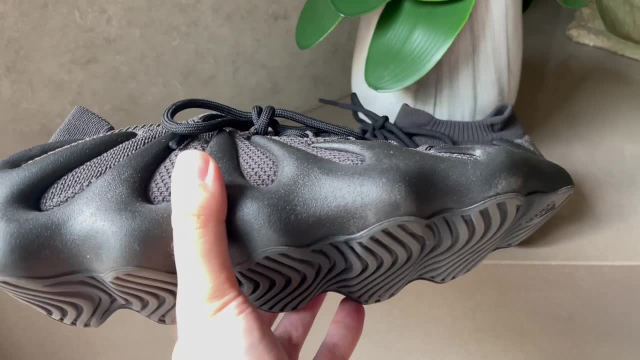 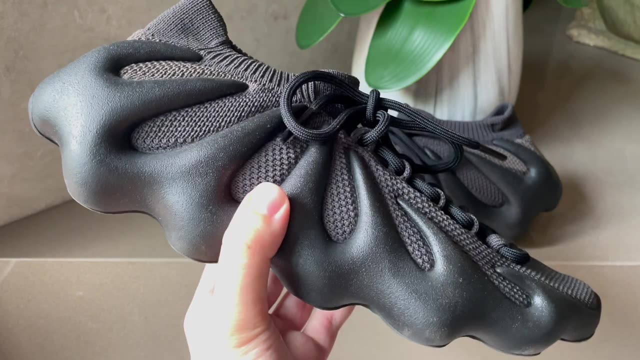 let me show you guys, the right shoe really quick as well, so you can see dirt marks again appearing on the same exact area. super durable and very comfortable. really have no complaints about these. so that is the up-close look on how they've held up after a little bit of wear. all right, everyone. 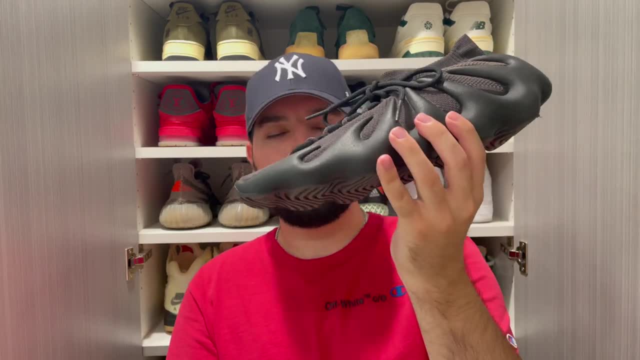 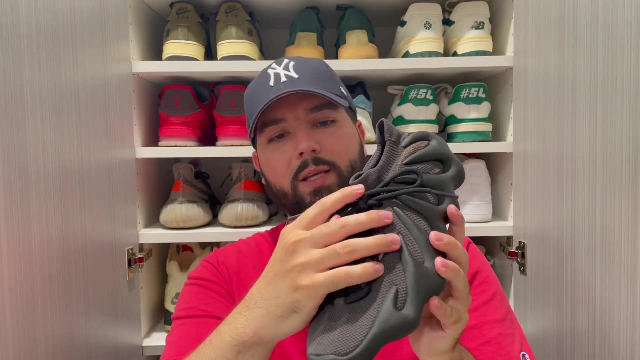 thank you so much for watching this video again. these are the ez450 dark slate. this was an update after two weeks of wear video. one thing i also want to mention is that i think these would actually look really cool with some white laces on them, finding some white rope laces like this. 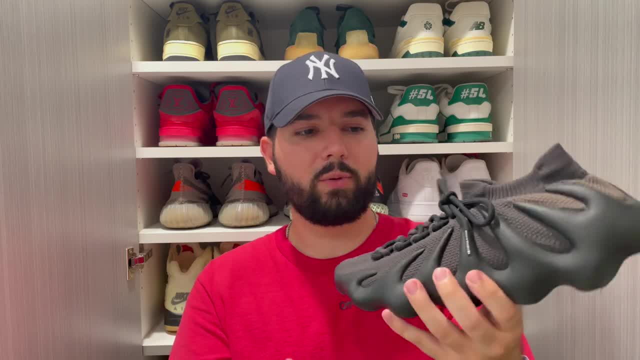 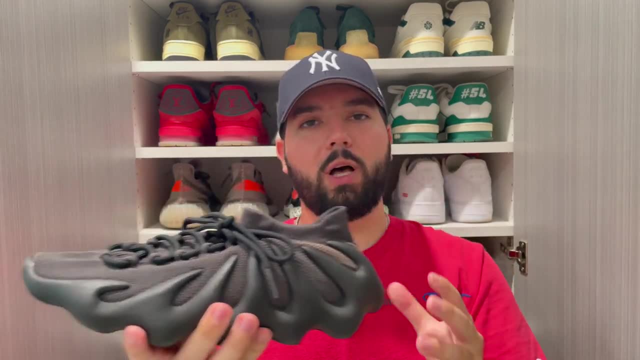 and throwing them on it would definitely give it a nice vibrant look. i might actually do that right now. i want that stealthy, you know look, but over time i might switch it up, make it a little bit different. but yeah, let me know your thoughts about the sneaker down below. i know a lot of people. 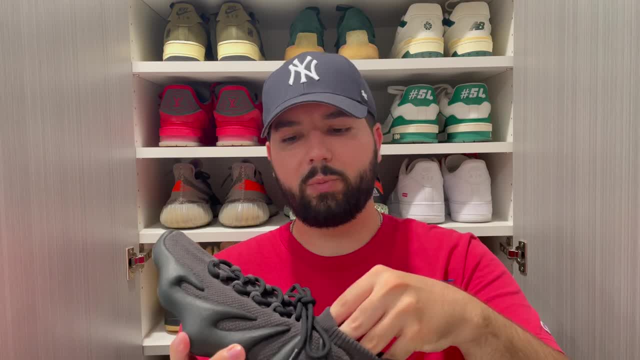 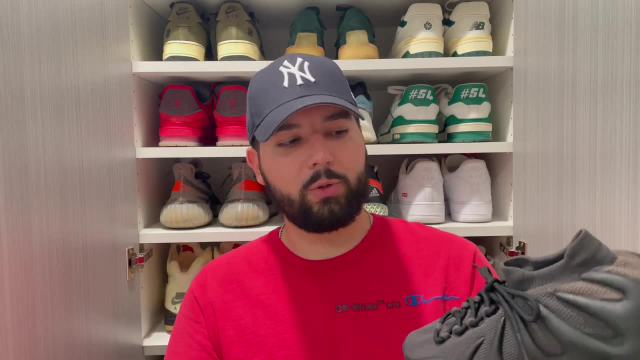 have differing opinions on these, one of my favorite sneakers of the past couple months, definitely something unique and something i like wearing out. if you've worn them and have a different type of feedback, i'd love to hear that as well. i'm always open to see you know. 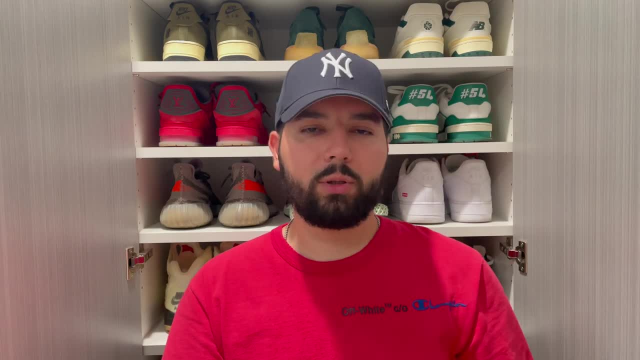 some of the things that i've seen in the past couple months, so i'm going to show you guys seeing what people think of these and other sneakers like that. so just comment down below. let's have a conversation. if you guys like this video, please make sure to like and subscribe for. more.